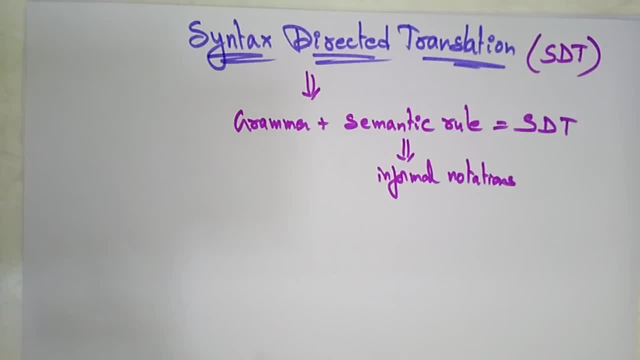 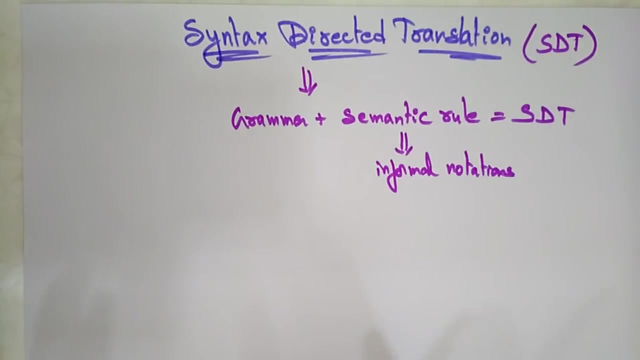 So that combinedly, you call it as a syntax direct translation. Okay, so you will understand why we are discussing the example, So don't be confused. So whenever they asked about what is a syntax direct translation, you need to tell that Grammar, along with some informal notations like semantic rules, you call it as a syntax directed translation. 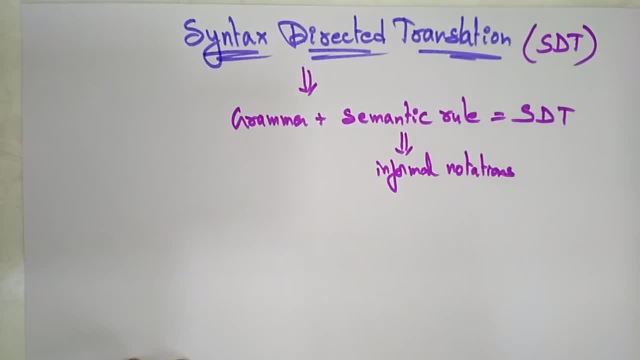 So in syntax directed translation every non-terminal can get zero or more attributes, depending on type of attribute. So just remember this point, Okay, so you will understand why you are seeing the example. So in syntax direct translation every non-terminal, So non-terminal, means you already know that. 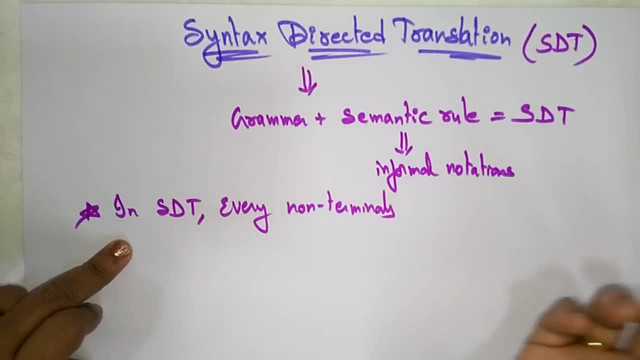 The capital letter alphabets. Okay, that you will see in the productions. So every non-terminal can get zero or more attributes. So each non-terminal can get zero or more attributes depending on the type of attributes. Okay, so in semantic rules, in semantic rule, attribute is a value. 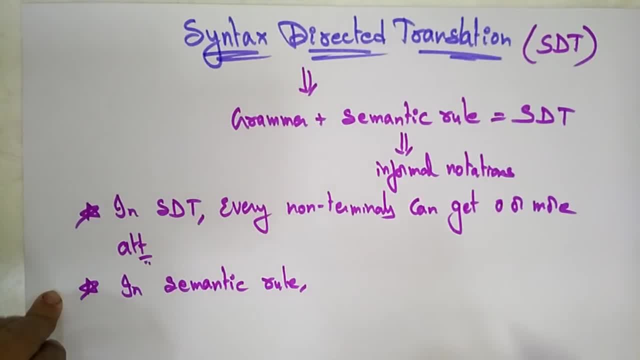 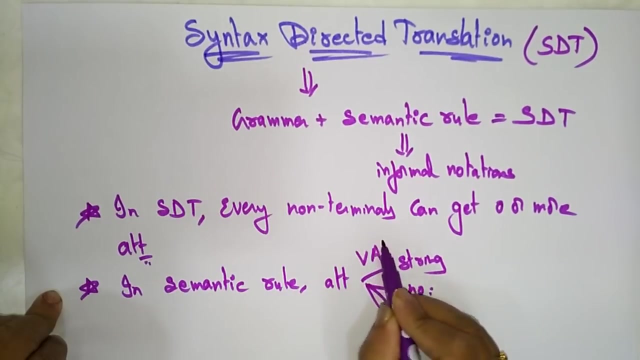 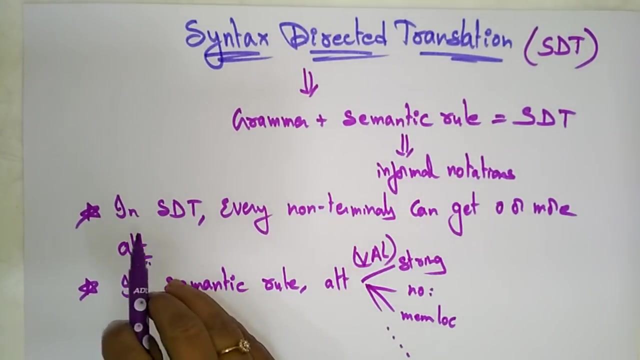 And can hold string, number or memory locations, whatever it may be. So this attribute can hold a string, numbers or memory locations, or whatever it may be. So we are representing it as a valve. The attribute can be represented as a valve. So in the semantic rule- So just remember this point- So in syntax, directed translation, every non-terminal can get zero or more. 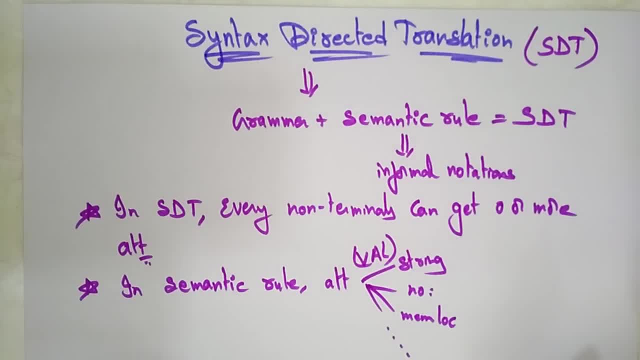 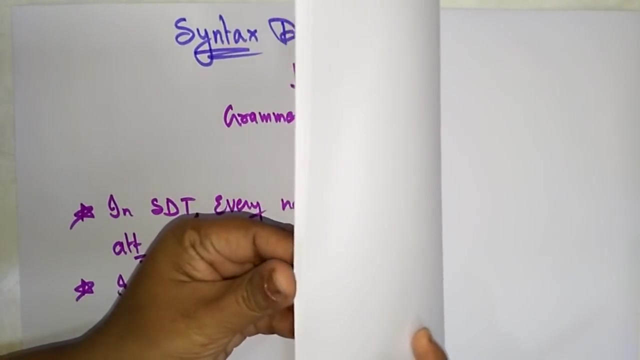 More σs can get zero or more attributes. That is support. type of attribute you are using: Okay, the integer. Whatever the type of attribute you are using, In semantic rules an attribute can be represented as a valve. Okay, so the values, nothing but the valves is nothing But the attribute. these attribute maybe a string, maybe a number. it maybe a memory location or whatever. 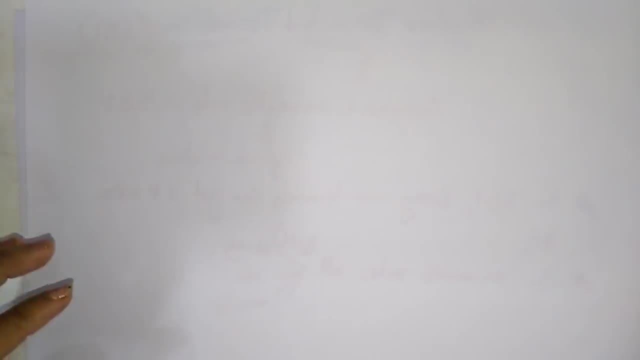 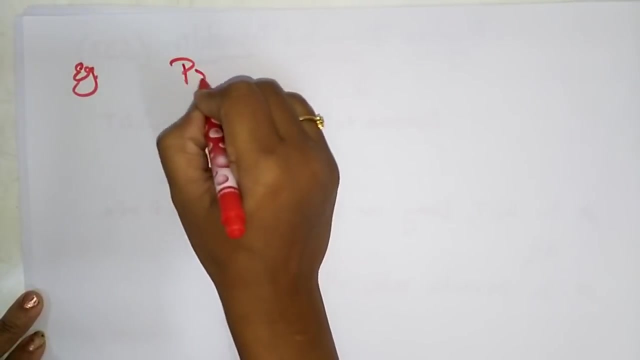 So now let's see the examples rules. you call it as a syntax directed translation. so what is that grammar and what are the semantic rules for that? let's see this here: the productions. production is nothing but the grammar, okay, and the semantic rule for that. 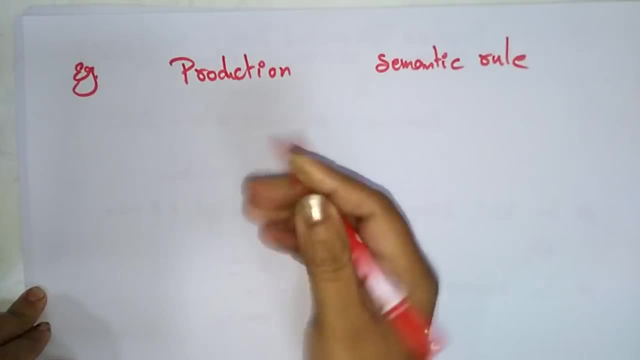 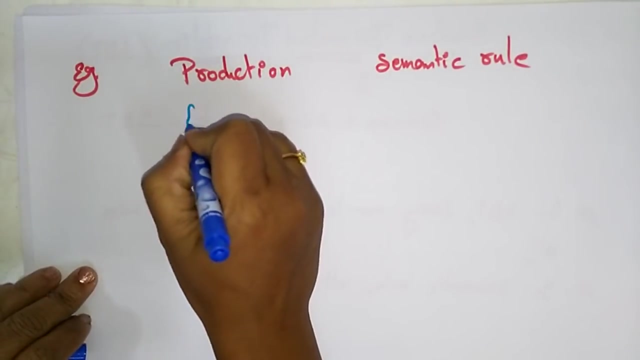 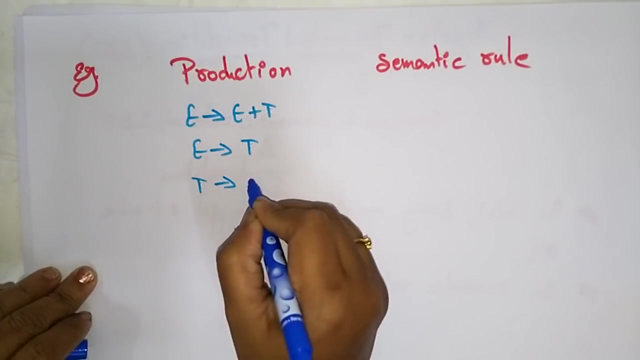 production. so combinedly you call it as a SDT. so just I'm taking the grammar here: e determines e plus T, e determines T, T determines. let's take these T into F, and T determines F, F determines number. these are the productions. so what are the semantic rules for these productions? the semantic rules are said, it is. 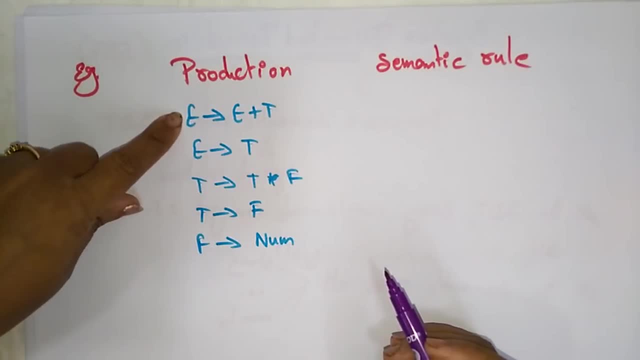 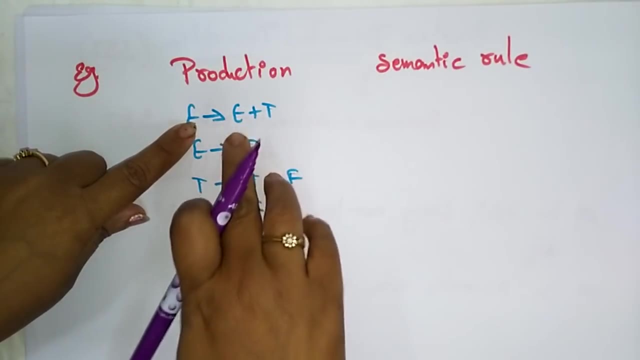 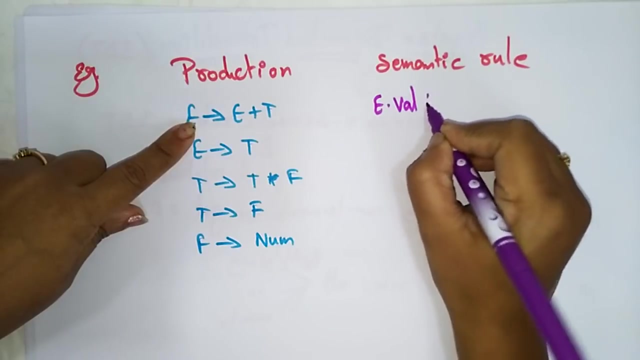 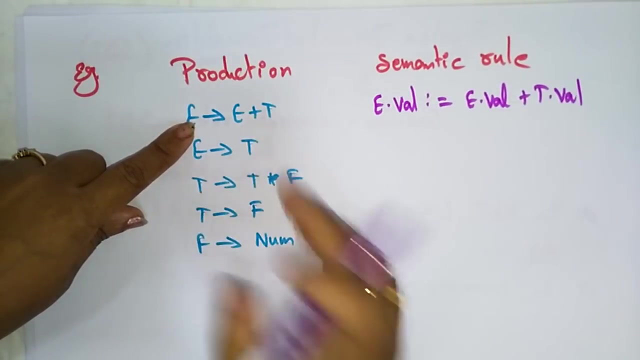 associated with an attribute. the non-terminal can get zero or more attributes, so that we know that. so this semantic rule here: these non-terminal will be added with an attribute: e dot valve value is equal to e dot value plus T dot value. so just simply add value attribute to that productions. okay, so it's because. 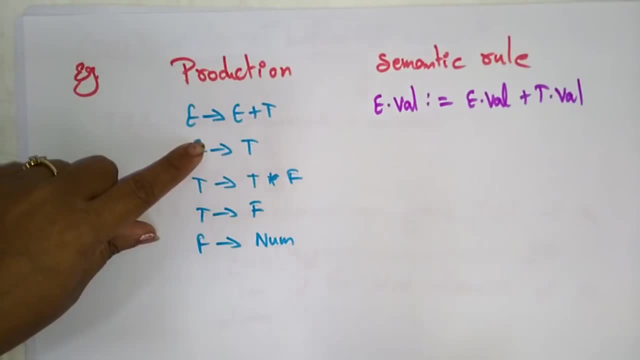 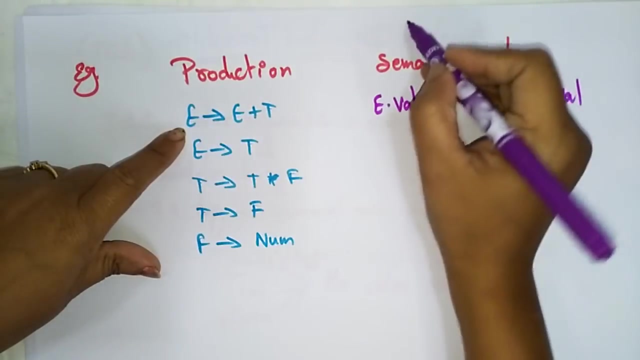 semantic rule is nothing, but it's an informal notation. it's just simply an informal notation, so you can add whatever the attribute name you want. you can add: okay, so this is a semantic rule. for this. productions means for this production. these are the actions. so this is a production and this is an action for that production, just remember. 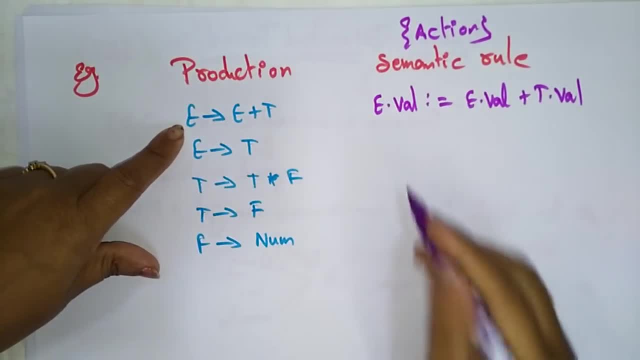 for each production there is an action, and here this sillcan. this action is: e dot valve is equal to t T dot valve. and T dot B, sorry, is equal to e dot W, QA, and T dot S is equal to t dot, and so for this action means e dot V is equal to e dot valve is given by I. so these factors which we have to explain, and here this action is B and Has it equivalent to t dot valve, and here this one can, for each action, E. 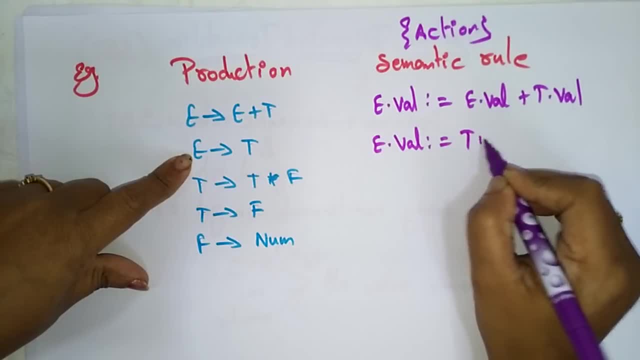 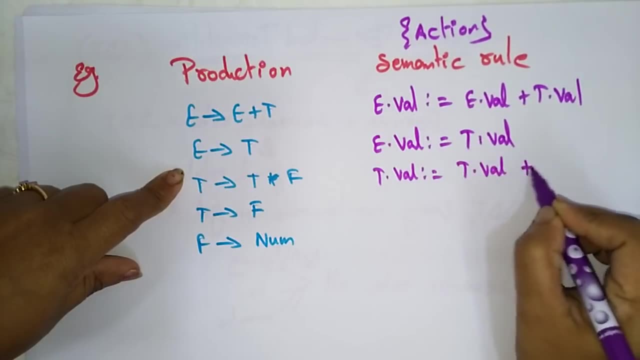 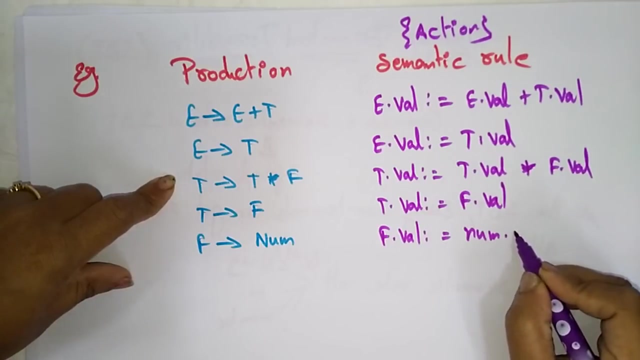 dot valve in simple and simple collection and you can see whether production and is equal to t dot val and t dot val is equal to t dot val. star, f dot value and t dot value is equal to f dot value. Finally, f dot value is equal to number plus. you have to write: 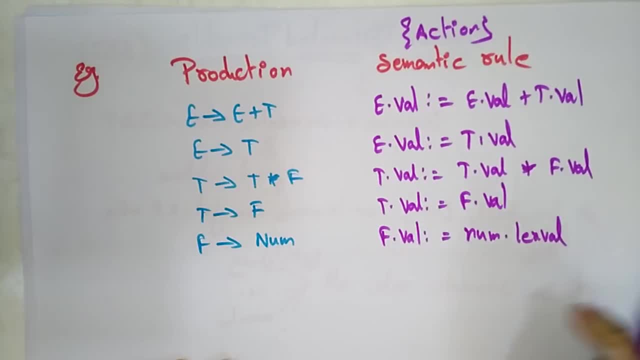 x values, l values, or you can take it as a lex value. So this is the example for SDT syntax directed translation. So here the num value is the attribute written by the lexical analyzer. So, attribute written by lexical analyzer. Okay, So this is an introduction.